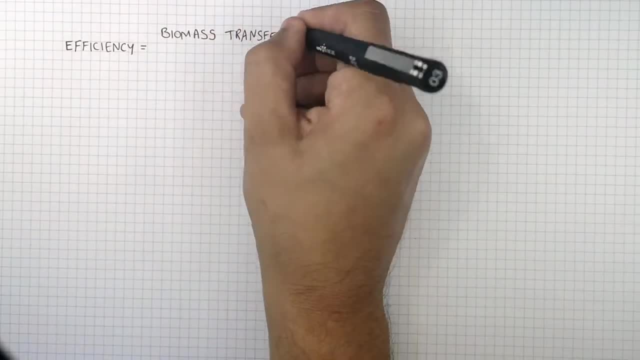 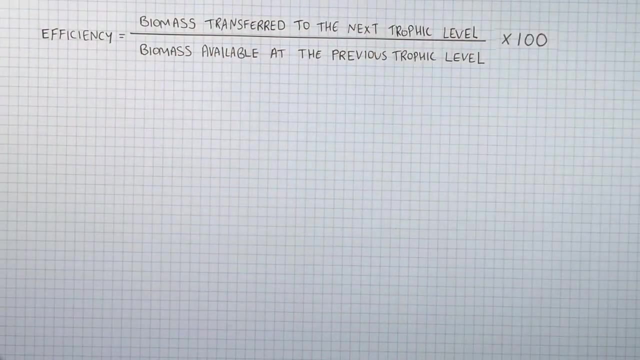 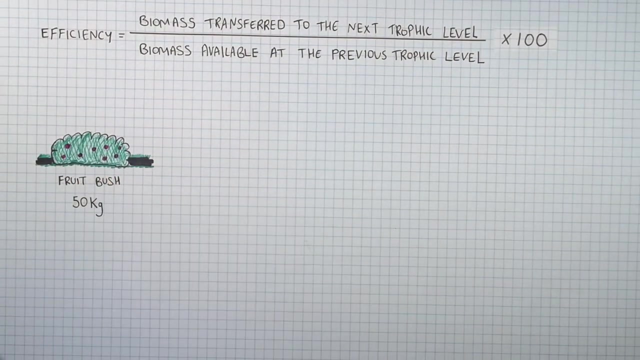 is efficiency equals biomass transferred to the next trophic level, divided by biomass available at the previous trophic level, multiplied by 100. This here is a fruit bush with a mass of 50 kilograms. So there is 50 kilograms of biomass. So there is energy stored. 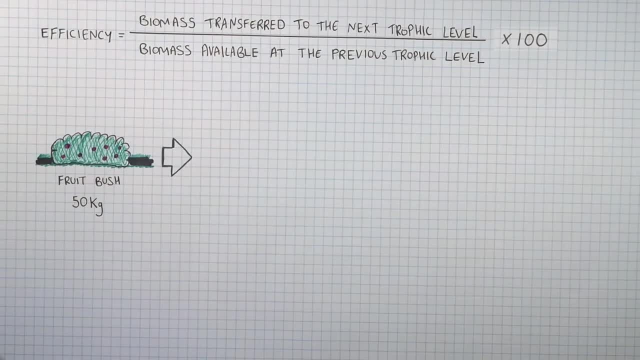 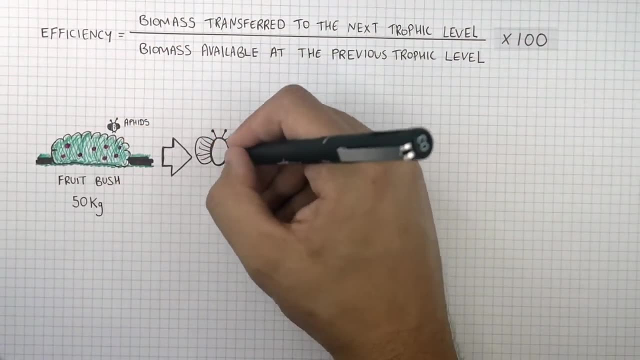 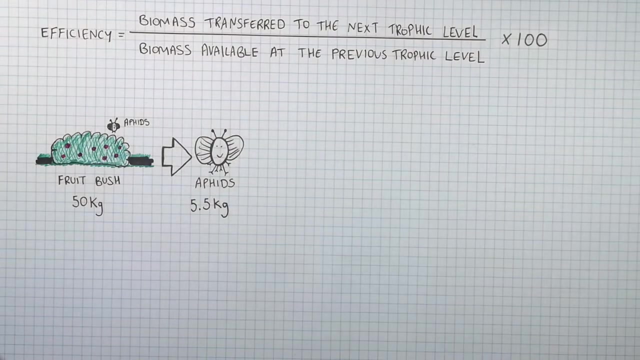 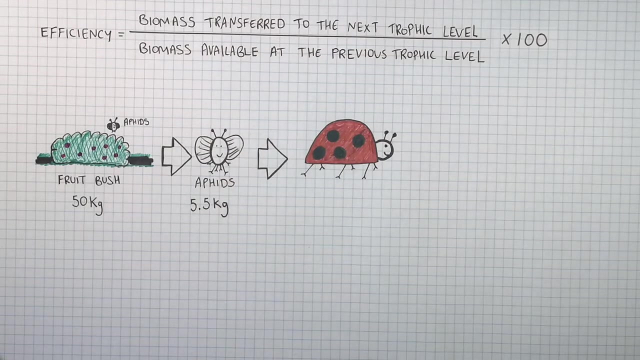 in the biomass of this fruit bush. Aphids feed on the biomass of this fruit bush, So 50 kilograms of biomass of this fruit bush is transferred to 5.5 kilograms of biomass stored in the aphids. Ladybirds eat the aphids. 5.5 kilograms of biomass of aphids. 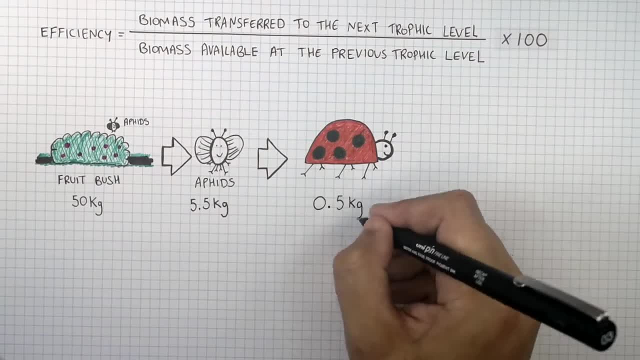 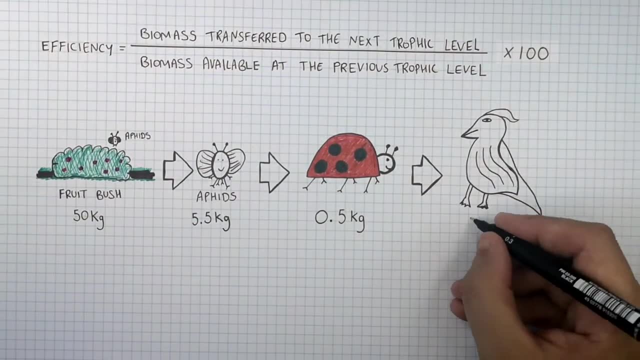 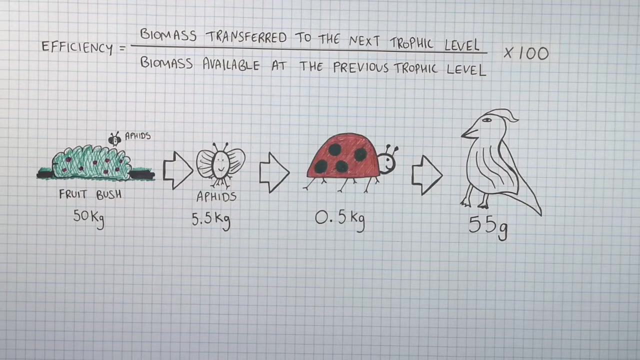 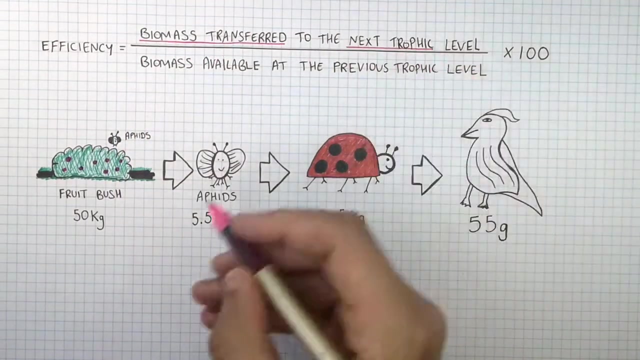 is transferred to 0.5 kilograms of biomass of ladybirds. So the 0.5 kilograms of biomass of ladybird will be transferred to 55 grams of biomass stored in the birds. So to work out the efficiency of energy transfer pushing the elimat to pressed toward the next trophic level between trophic levels, you must do. 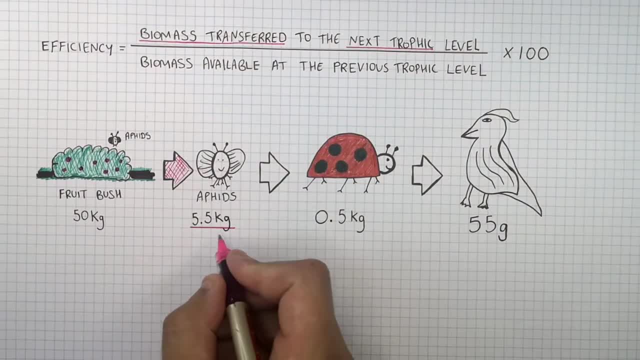 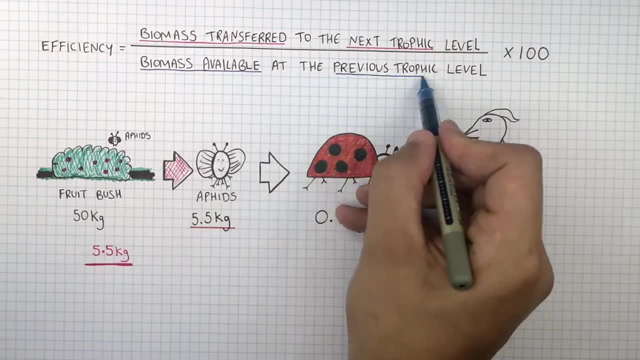 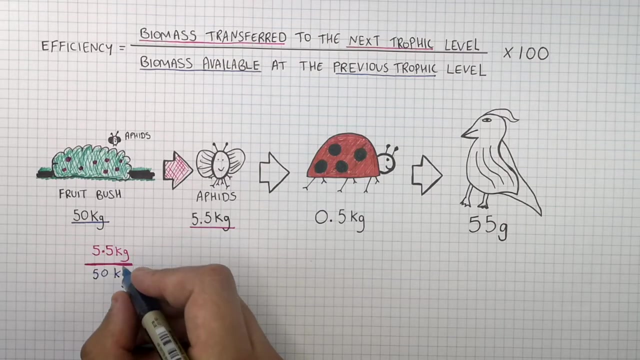 the biomass transferred to the next trophic level, Which is in this case. In this case, the aphids have a biomass of 5.5 kilograms. so you do 5.5 kilograms divided by the biomass available at the previous trophic level, which is 50 kilograms: 50 kilograms of biomass stored in the fruit bush. 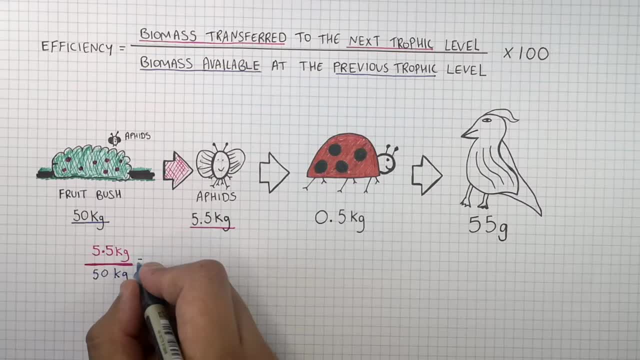 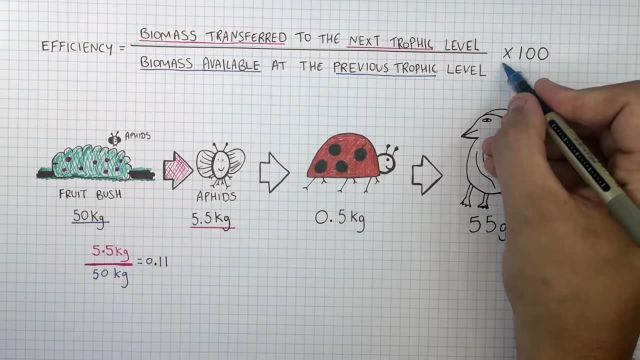 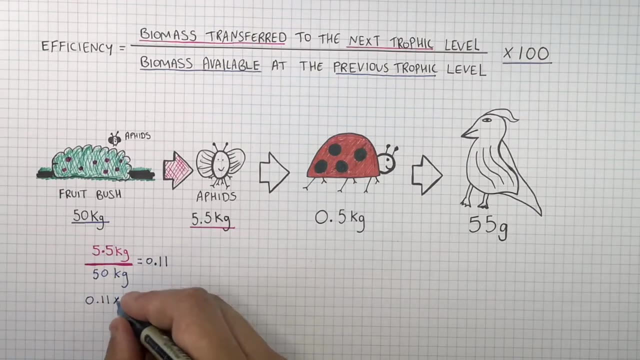 50 kilograms of biomass stored in the fruit bush, which equals 0.11.. So you must multiply 0.11 by 100.. So the efficiency of energy transfer between the fruit bush at the first trophic level and the aphids at the second trophic level is 11% efficient. That means that 89% of the energy 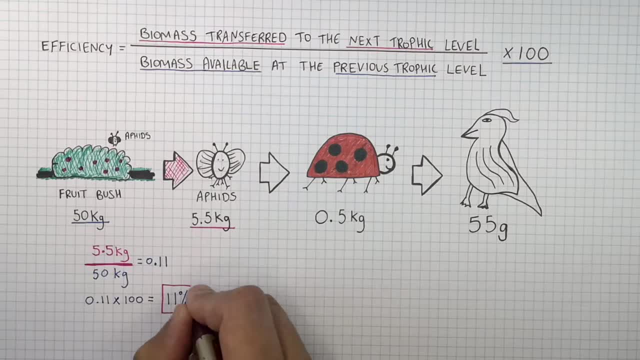 stored in the biomass of the fruit bush is transferred to other energy stores. So 5.5 kilograms of biomass in the aphids at the second trophic level is transferred to 0.5 kilograms of biomass stored in the biomass of the ladybirds in the third trophic level. So to calculate the 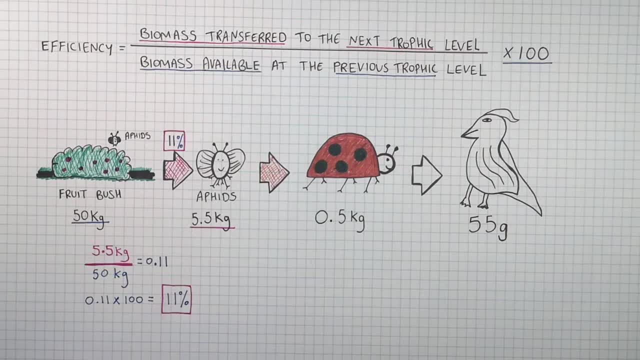 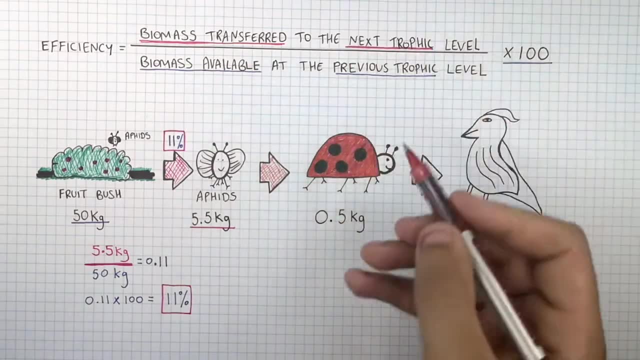 efficiency of energy transfer between these two trophic levels, you do 0.5 kilograms, which is the biomass transferred to the next trophic level, Divided by the biomass available at the previous trophic level, which is 5.5 kilograms of the aphids.